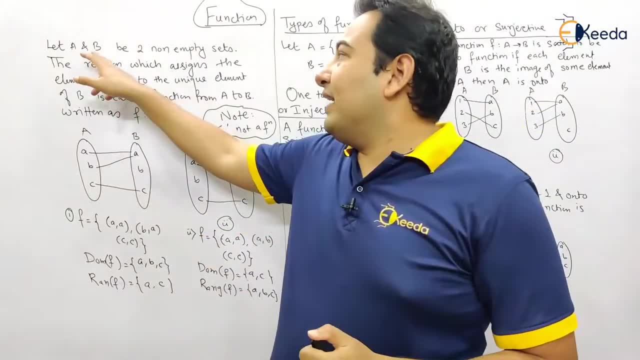 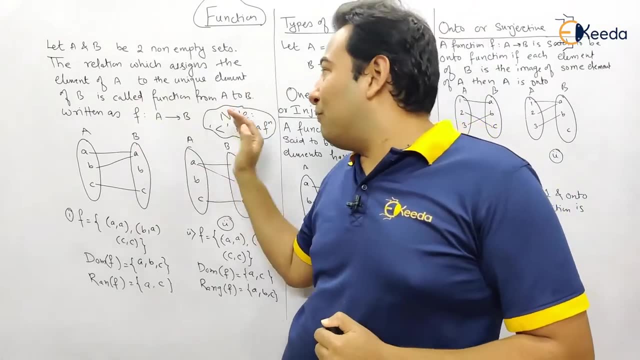 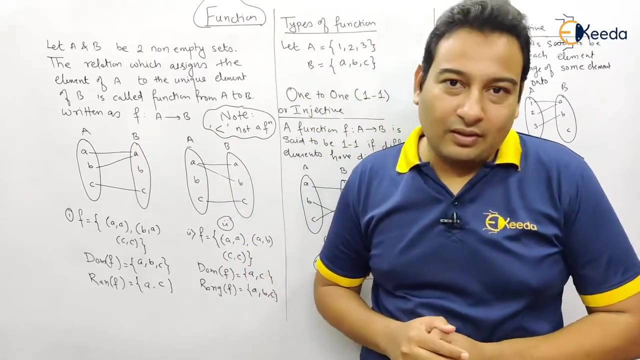 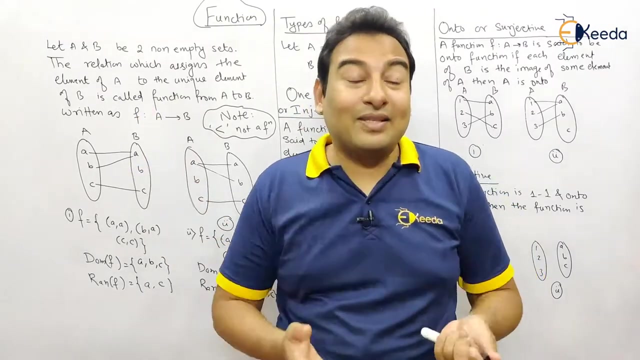 So let me read it. Let us try to understand. It defines the element of A to the unique element of B is called function from A to B and it's written as F to dots A to B. Read the definition again and try to understand. This is your textbook definition that if comes in the exam you need to write it down. So you need to remember the definition. 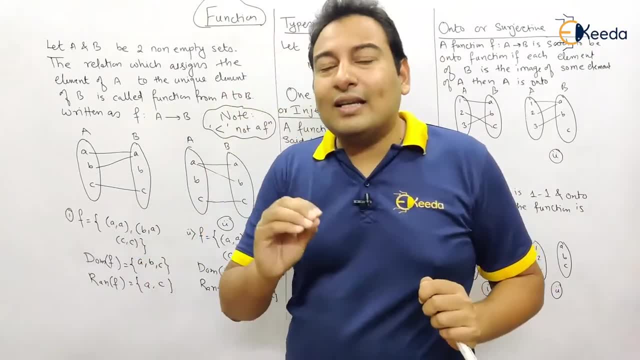 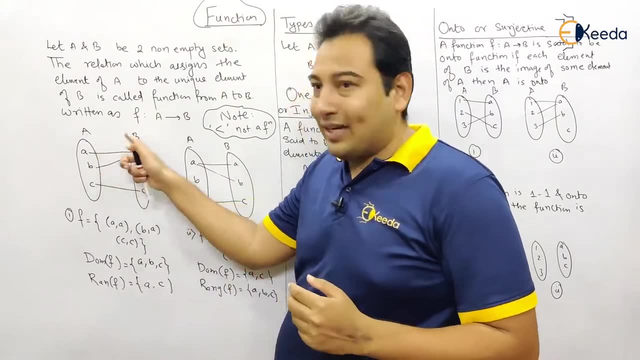 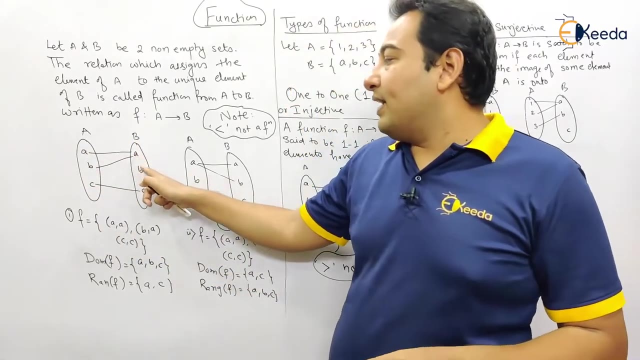 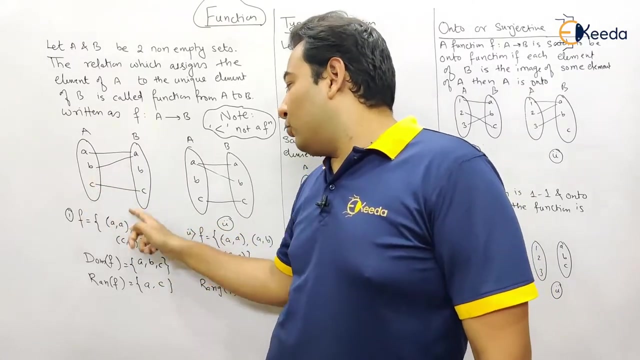 I'll explain you, Don't worry. Don't worry, It's a very simple thing, What the definition says. See, first of all, if it is a relation, then there has to be a subset of A cross B. It has to be two sets Here. the first set, A, contains the elements A, B, C. The second set, B, contains the elements A, B, C, And there is a function given and it is saying: from A to A, B to A and C to C. 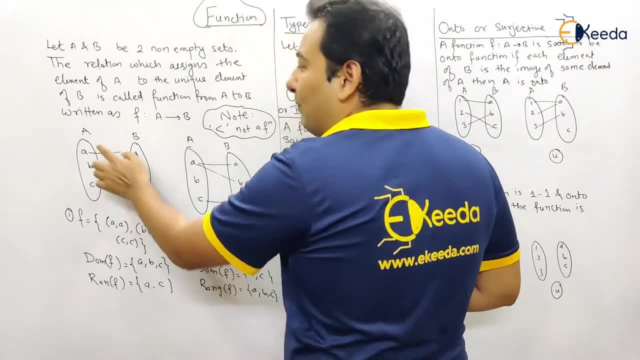 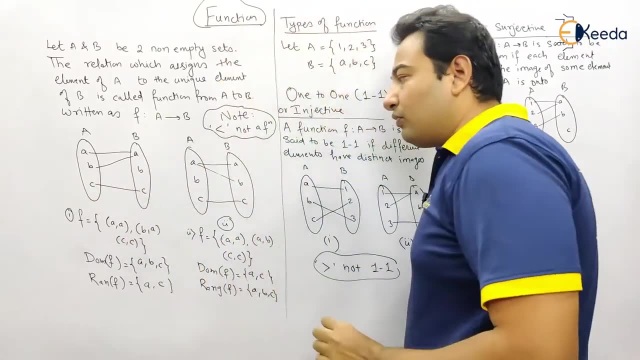 So this is the function given and it's a function from A to B, or you can say it's a relation from A to B and it is given. We have written in this format What the function says from each element of A. There should be only one link. 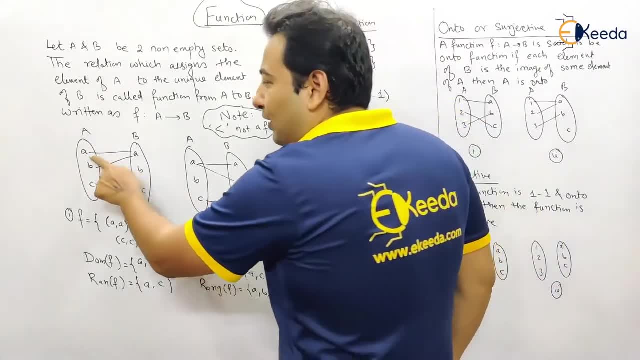 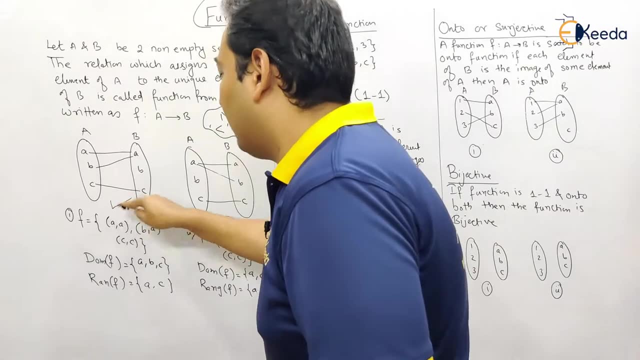 From every element of A. there should be only one link here. From A, there is only one link. From B, there is only one link. From C, there is only one link. Therefore, it's a function. If you observe the second example: from A there are two links. 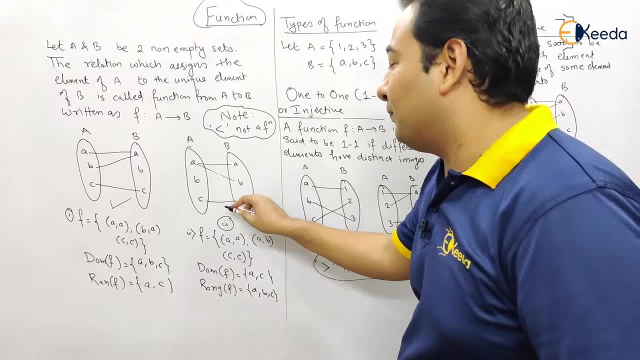 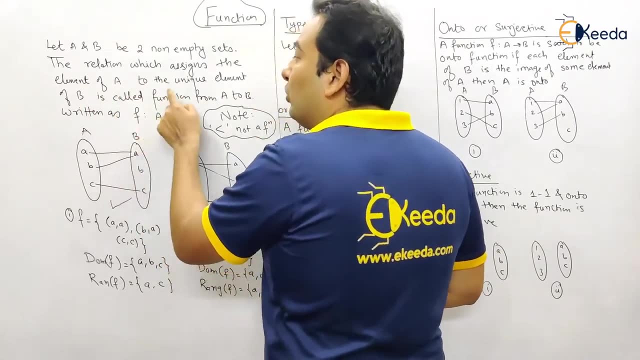 From A. there are two links. Therefore it's not a function. Is this clear? Now let us read the definition, which assigns the element of A To the unique element of B. See this element A is assigned to the unique element A. 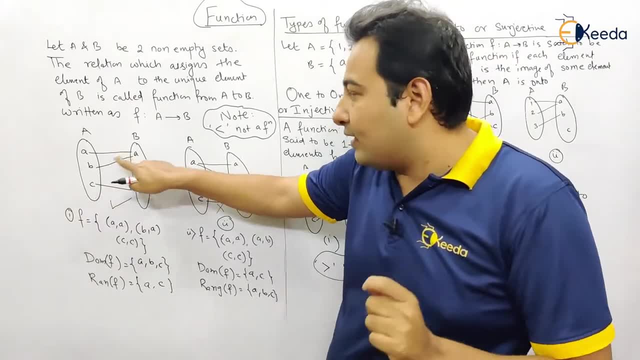 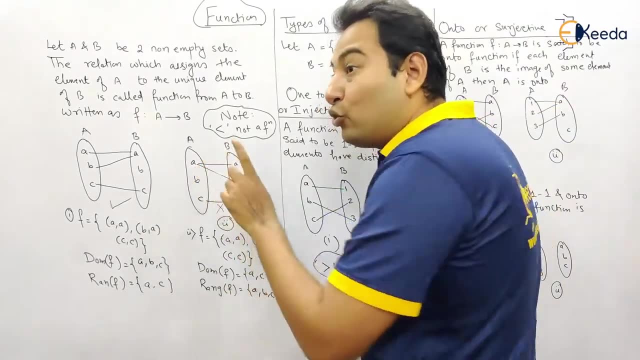 This element B is assigned to the unique element A. This element C is assigned to the unique element C, Therefore it's a function, Whereas this element A is not assigned to the unique element. This element A is assigned to two elements: A and B. 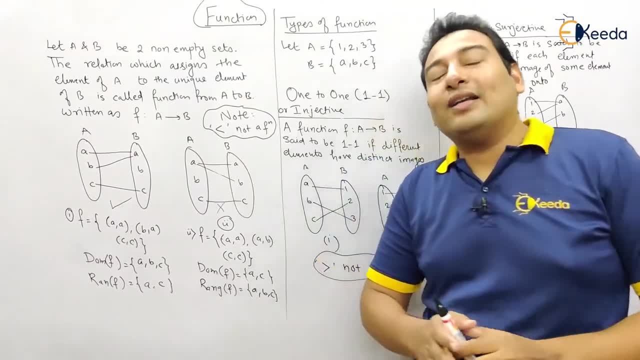 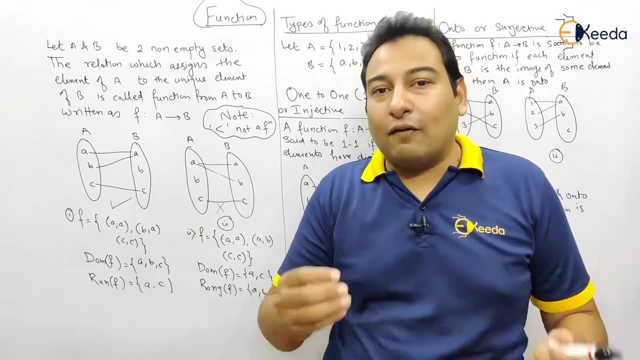 Therefore it's not a function. Is this definition clear, publique on or in a simple language? there should be only one link. If there are two or more link, it's not a function here, it's a note is written if you get something like this: 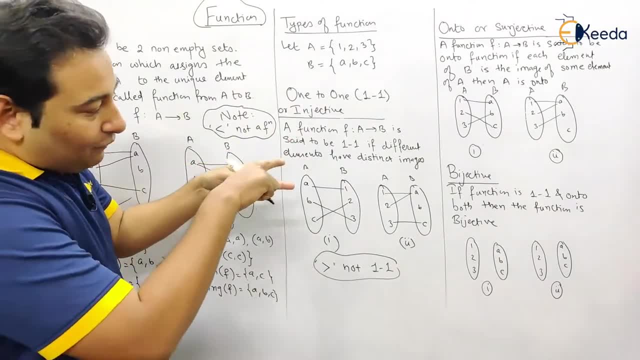 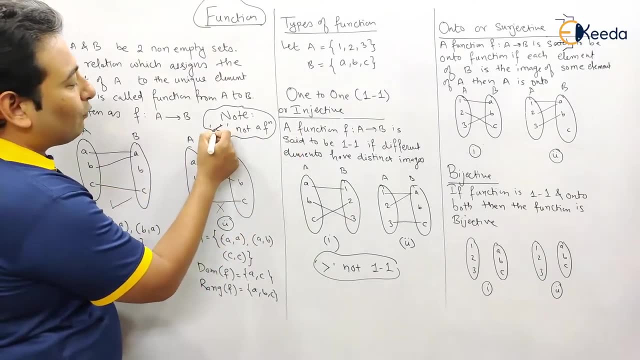 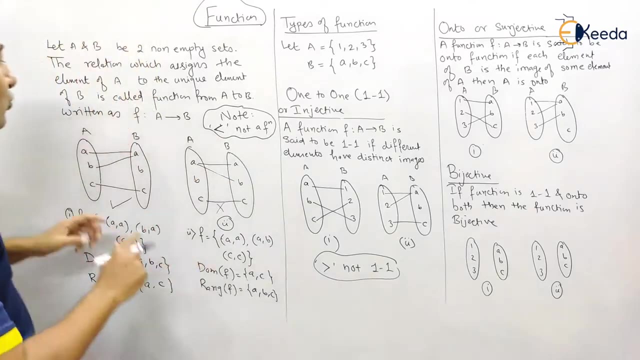 it's not a function. that means from one. if there are two or more than two, then it's not a function. for the sake of remembrance, for remembering it, you can remember this sign. if this is the sign from one there are two or more elements, it's not a function. so this is the definition of function. 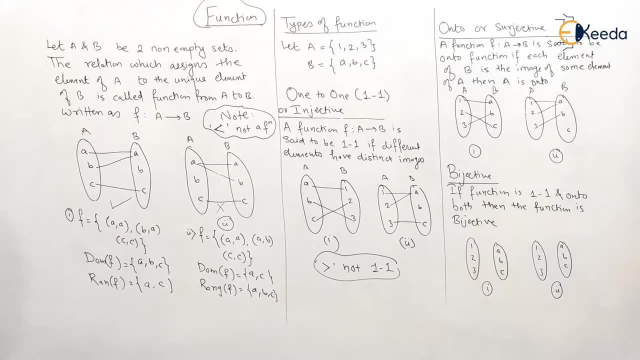 here we have taken two examples and we check which is function and which is not a function. next, there are two concepts. one is called domain and one is called range. what is the domain of the function? for writing down the domain of the function, all the first part of the, your element. 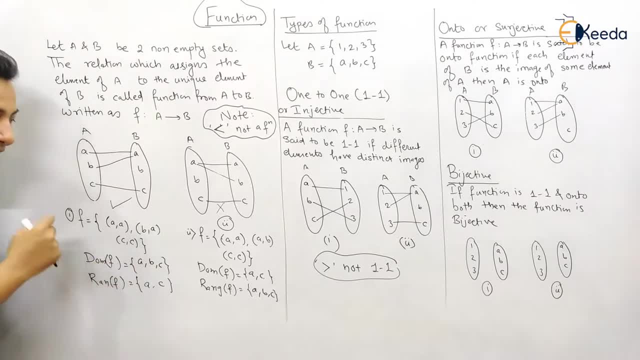 see here, a, b and c will be the part of the domain and the second element will form the range: a, a and c. so a- c is the range. is this clear? what is domain and what is the range? domain means the first elements of a function- a, b and c- and range means the second element. here, also, the first element is a- c and the second 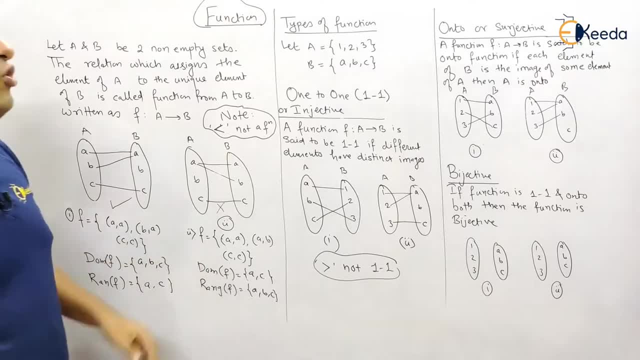 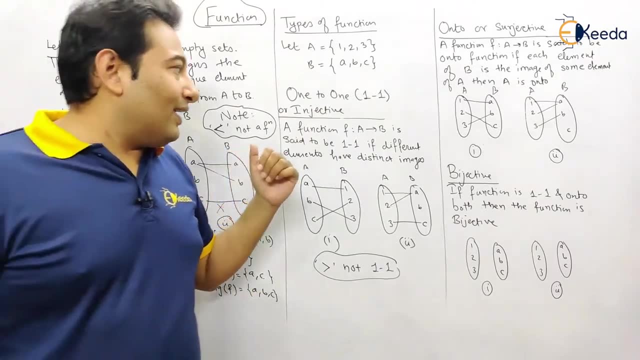 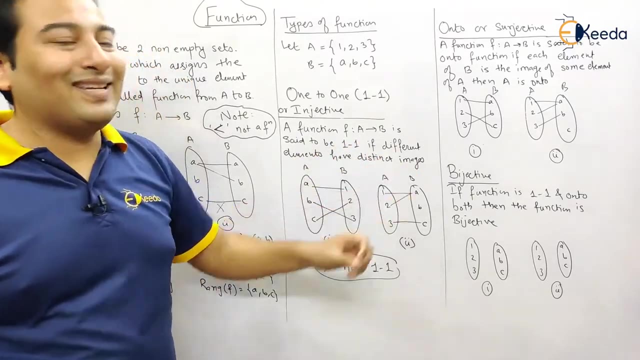 element is a, b and c, so domain and range. let us move on and let us discuss what are the different types of function. the first function is one to one, very important function, and the function says: is sample to be one to one if different elements have distinct images. that means that means, in short: 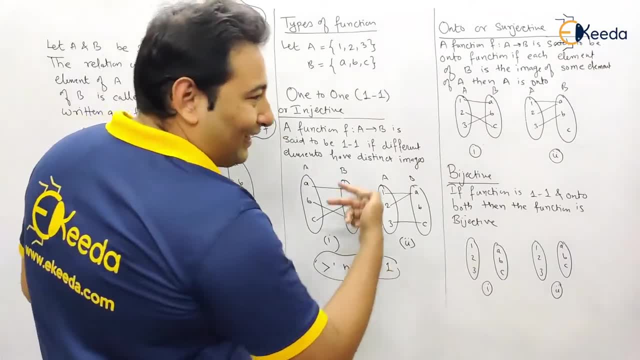 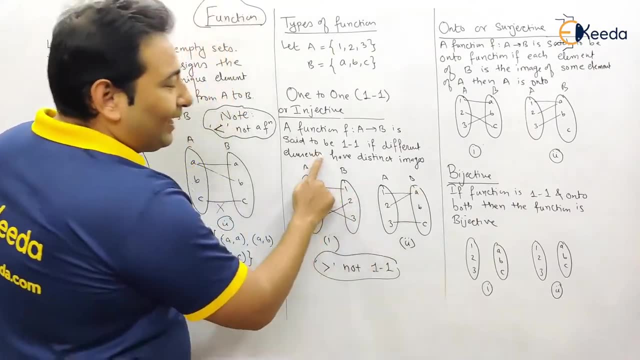 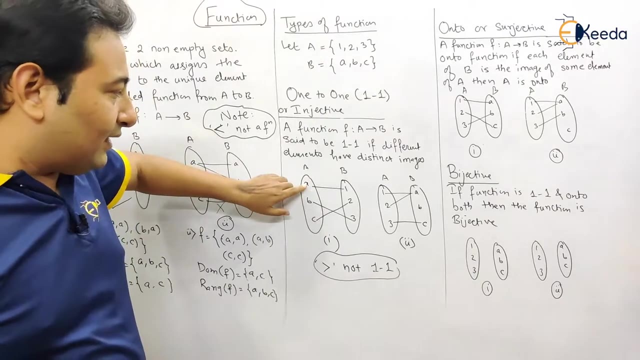 if you get something like this, it's not one to one. that means, see here, we're getting something like this. if the el, what the definition of one to one says, if the elements are different, it should have different images. see here this: this is: this element has this image. this element has this. 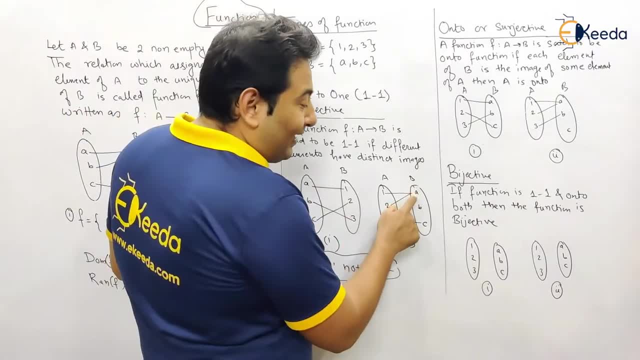 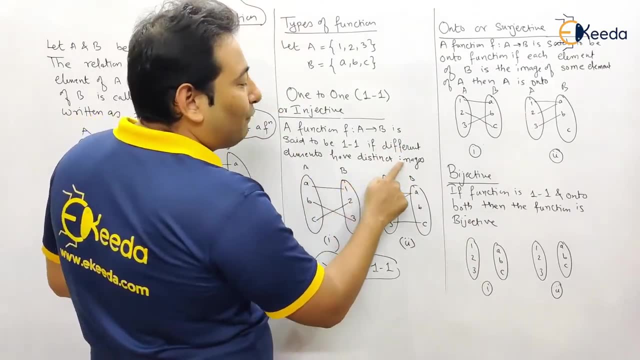 image. this element has this image, but here the problem is this element is an image of two elements, so which is not allowed. so what are the definition saying different elements must have different images. see, the elements are different, so their image should be different, one and two must. 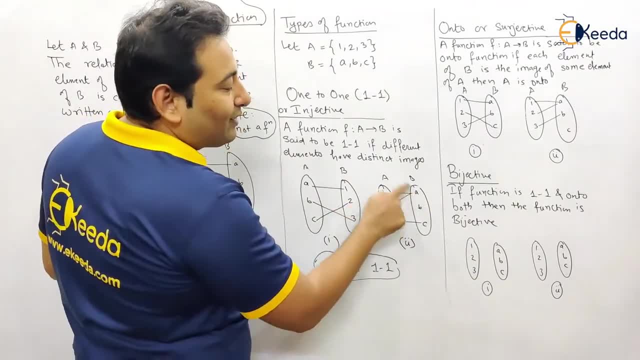 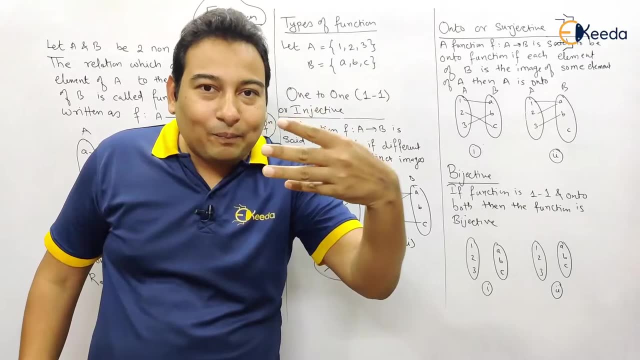 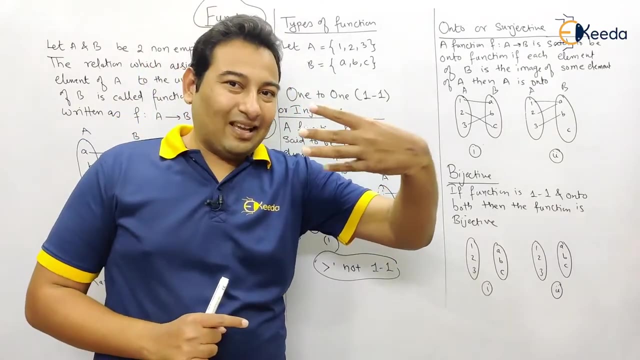 have different images, but problem is one and two is having the same image. in short, let me give you the trick. in short, if you get something like this: 2, 3, then it's not 1 to 1. that means at one point if two or three or four are meeting, then it is not one to one. is this clear? 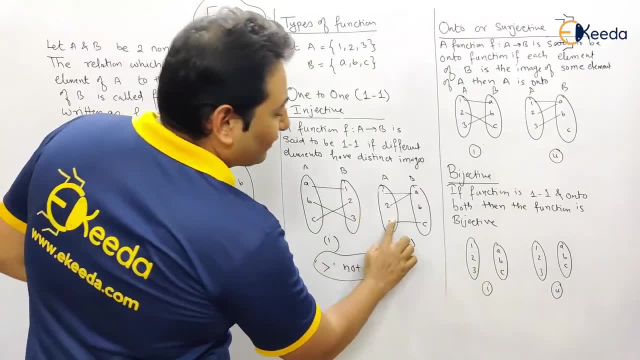 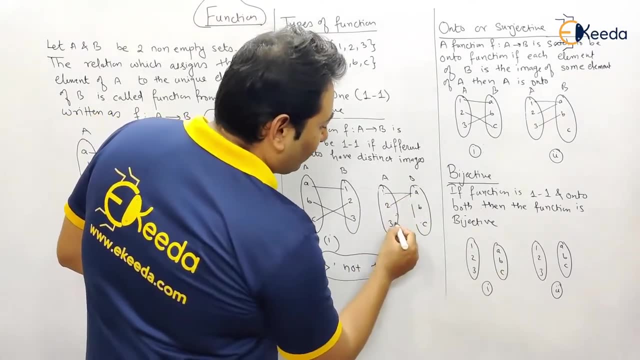 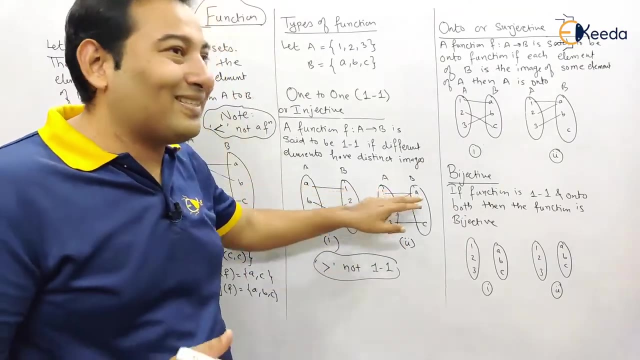 a at this point, two links are there. suppose this may be also possible. this is not. this is also not one to one. is this definition clear? if the elements is different, its image should be different, but here two different elements are there, but their image is same. it's not one to one. or in short: 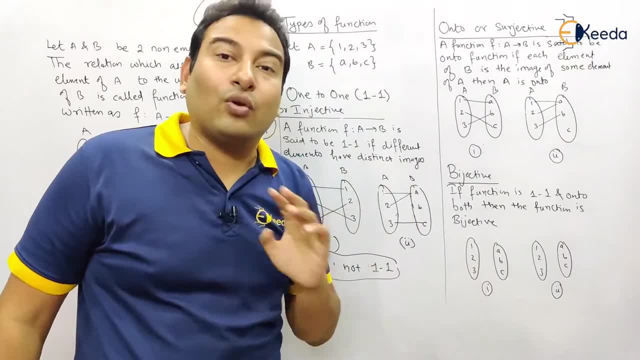 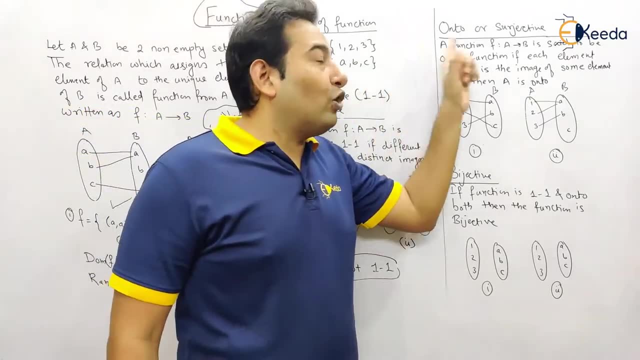 if this is the case, it's not a function of one to one, then it's not a function of one to one. if this is the case, it's not one to one, let us move on and let us discuss the next. that is onto one to one is also called injective function. next is onto. onto is also called surjective. 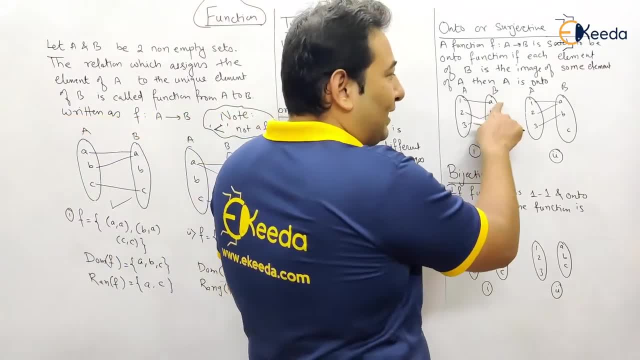 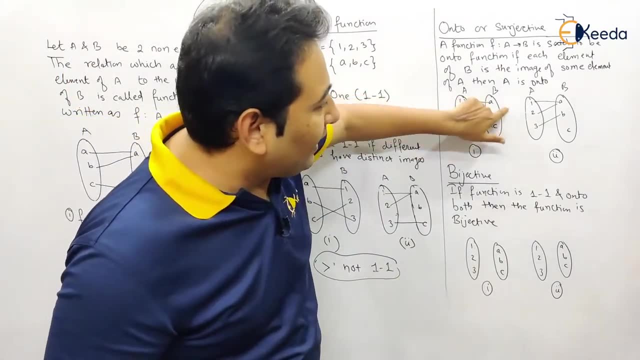 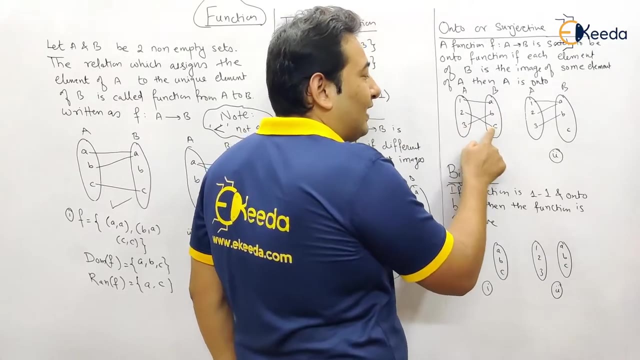 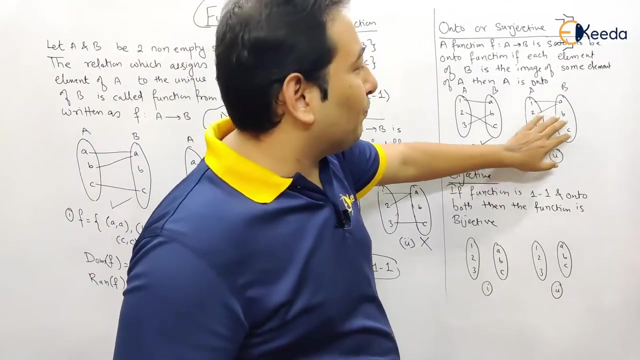 if every element of b has some element in a, then it is called onto see here: a, b, c. every element of b has some element in a. a has some element one, b has some element three, c has some element two. therefore it is onto. but whereas this is not onto, why? because this is obviously a function. 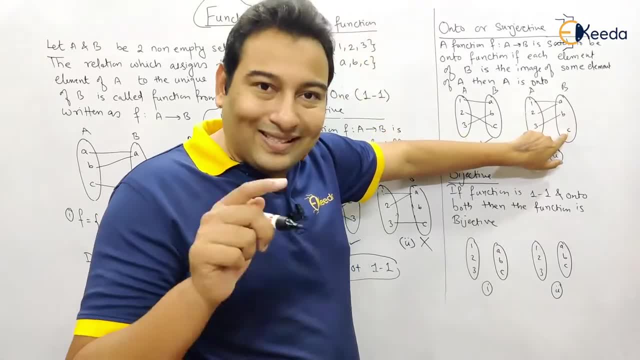 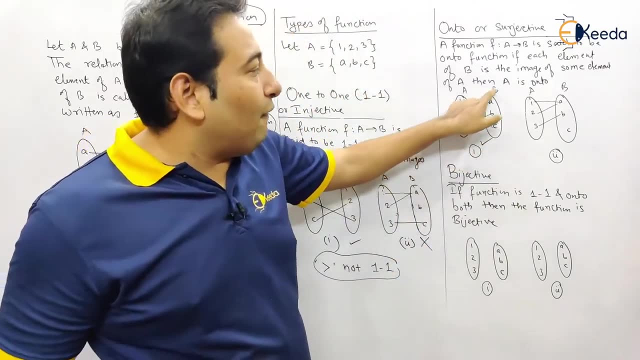 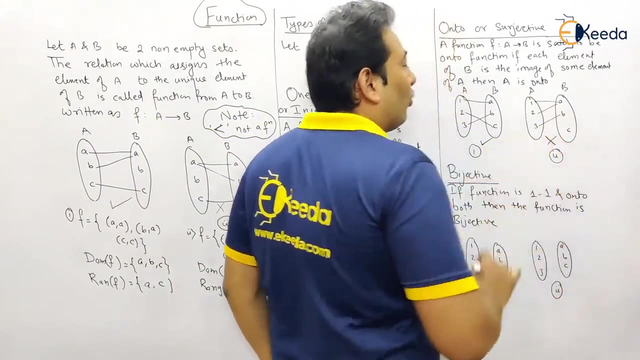 but it is not onto function. why? because for c there is no a, there is no element in a. so what do you mean by onto function? onto says every element of b must have some element in a. here for c we don't have element in a, so therefore this is not onto. 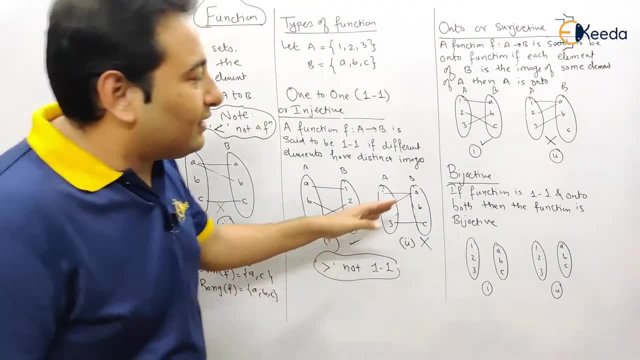 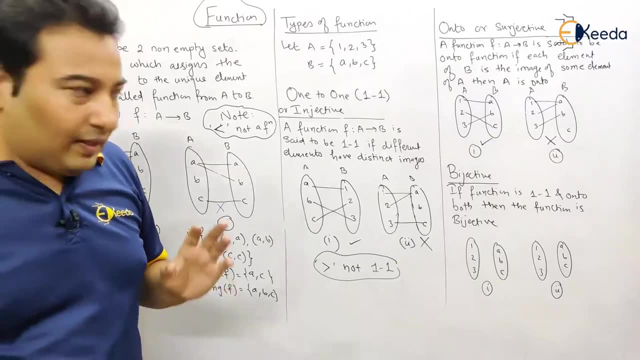 is this clear? and the last is bijective. when the function is bijective, if the function is one to one and onto both, then the function is said to be bijective. so let me write it down for you, examples here. first of all. first of all, it must be a 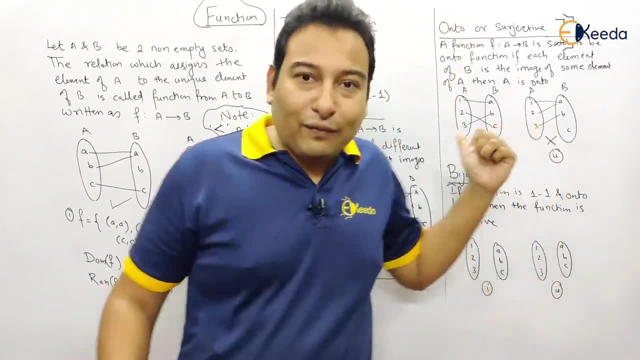 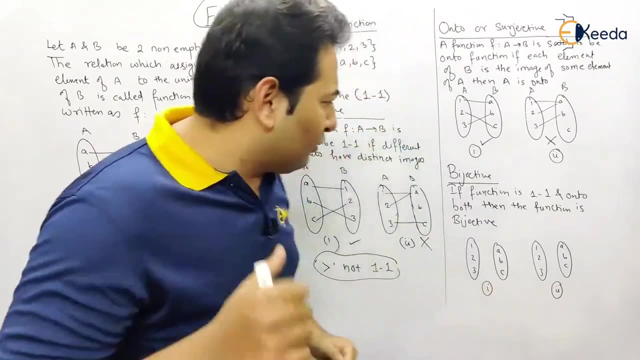 function. if must be a function, then only we schauen to check whether it is one to one, onto or bijective or not, because if it's not a function, no need to check. we can't check its type if it's not the function right. so first of all it has to. 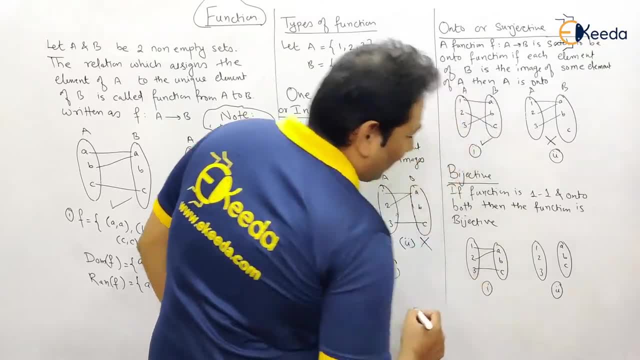 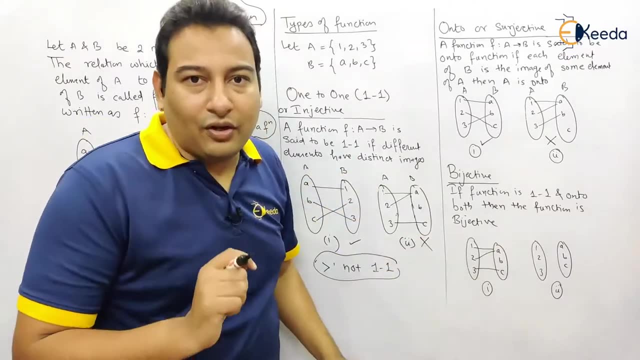 be a function. so me write it down, this: please tell me whether it's a function or not. it's a function, why, if you're not getting this particular sign, then it's a function. what about this one to one? is it one to one? no, it's not one to one because 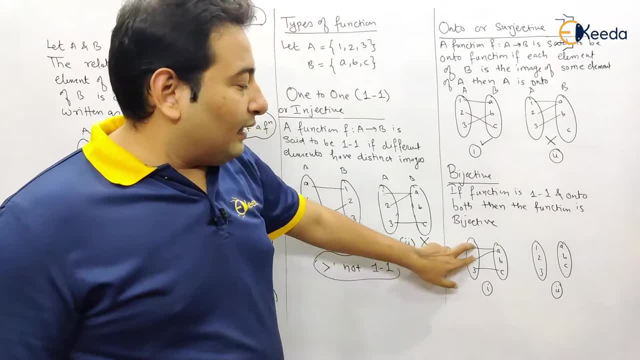 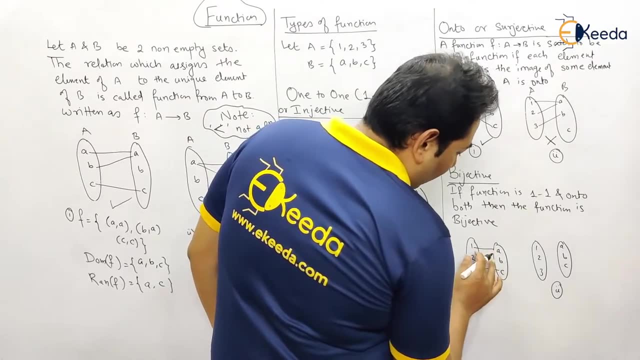 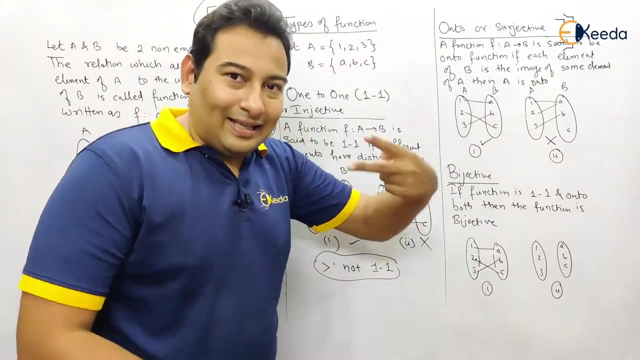 there are two lines meeting at the same point. it's not one to one. so we are writing down the example of bijective. so let me write it down something like this: yes, it's bijective, why? first of all, it's a function. there is nothing like this symbol, this sign. therefore, it is one. 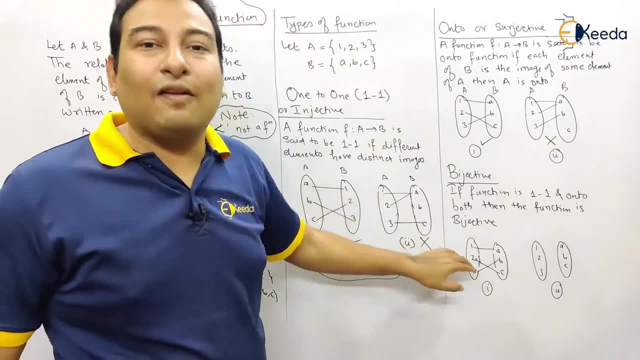 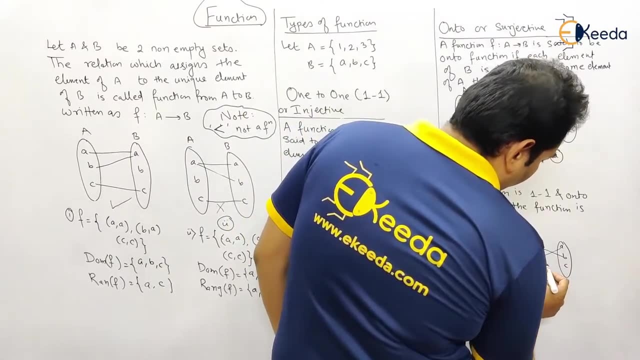 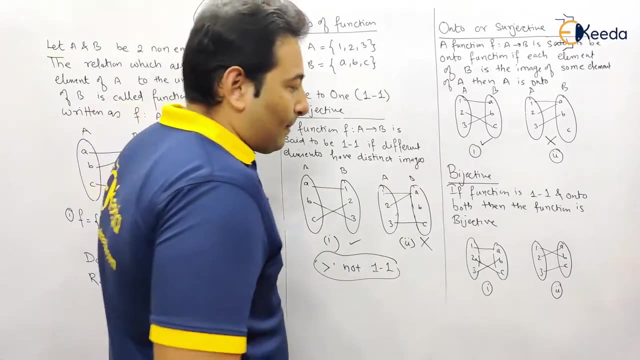 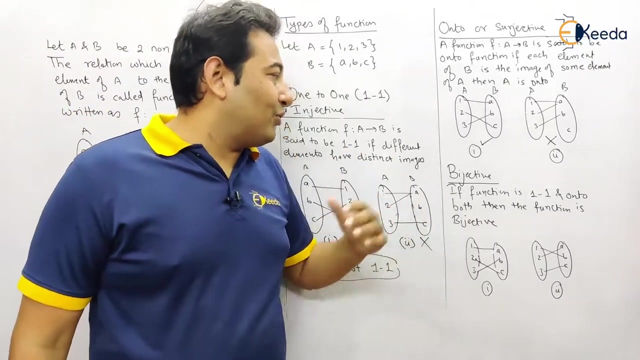 to one, and for every b we should have some a. therefore it is on two. therefore the function is bijective. again, this function is also bijective. is this clear? so we discuss the concept of one to one on two and bijective both, and whether it's a function or not in the same video. let us discuss few more. 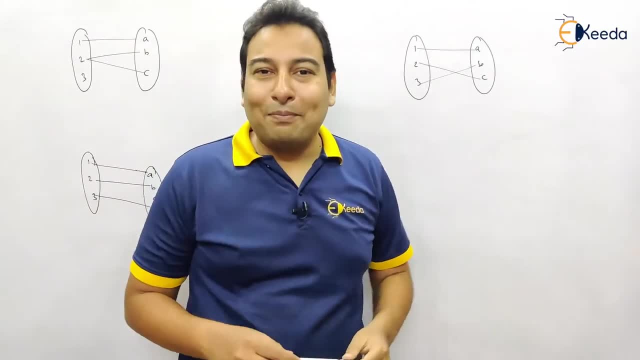 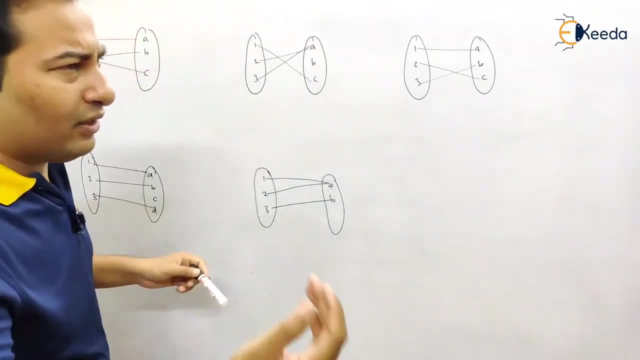 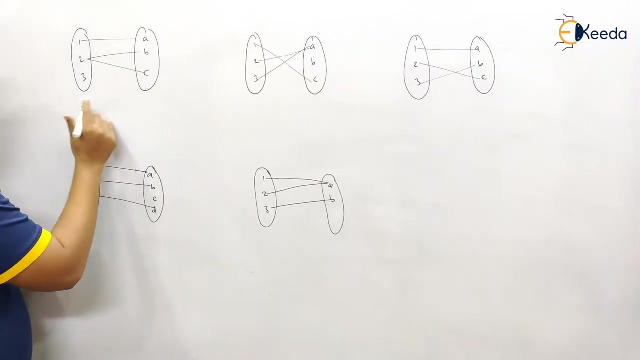 examples so that the topic will be very clear to you. few examples are written on the board. now we'll check which one is one to one to one bijective function or not. so let us start see here what is the first case this is not a function. why it is not a function. it is not a function. why? 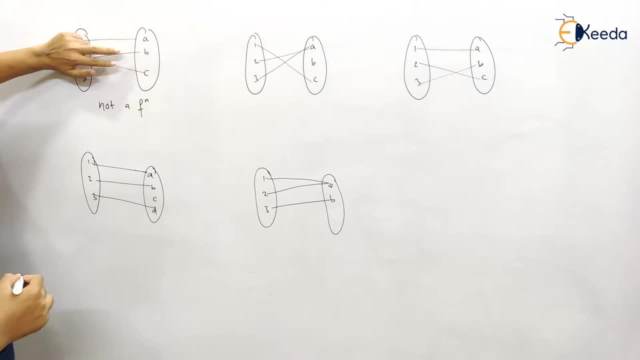 see here, from two. there are two links. so what is the definition of function? from every element there should be only one link. if there are two or more links, then it's not a function. since it is not a function, no need to this, we can't discuss. 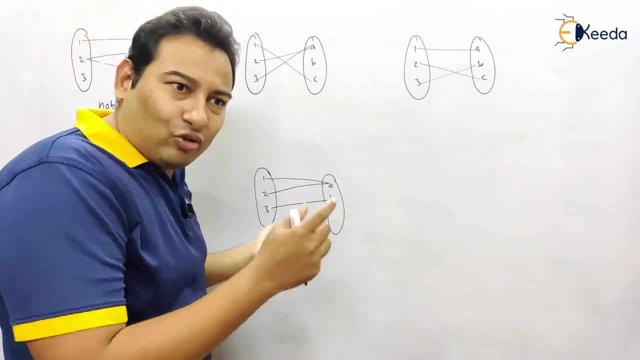 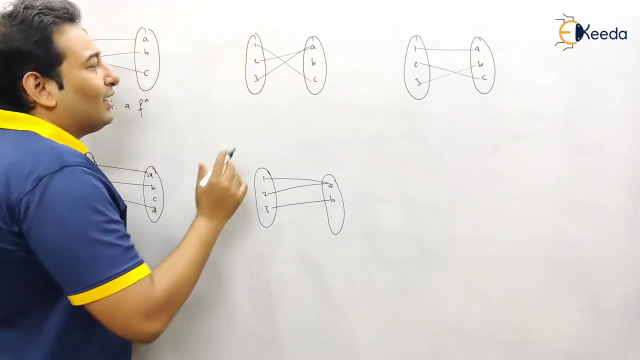 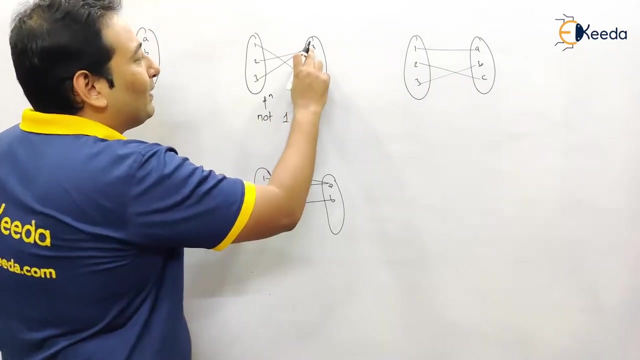 whether it is one, one on one, two and so on. first of all, it has to be function, so that after that we can check whether what is the different time. let us move on. it's a function, first of all. it's function, not one to one. why it is not one to one? because two and three have the same. 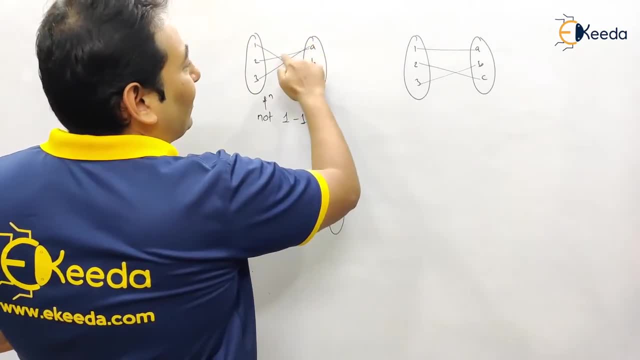 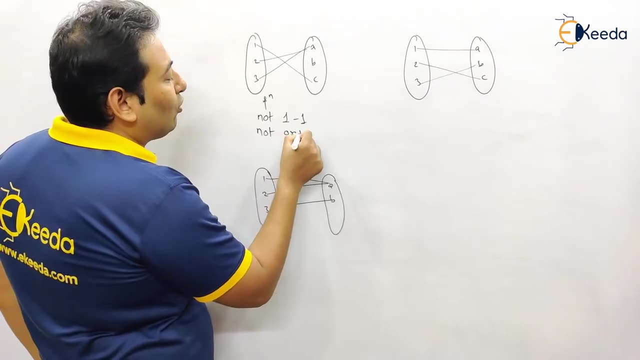 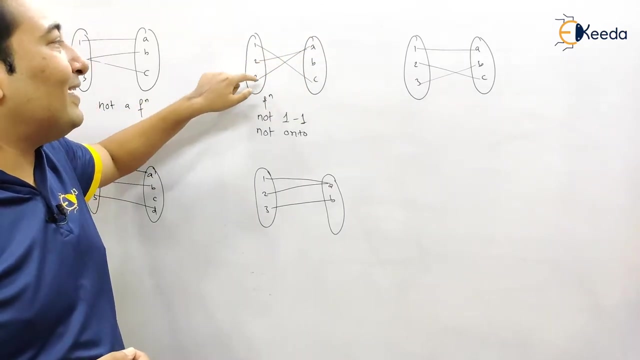 image. in short, at a there are two links which are meeting. therefore it's not one to one and as well as not on to. why not on to? because for B, what is the definition of one to? every element of B must have some element in a for B there.